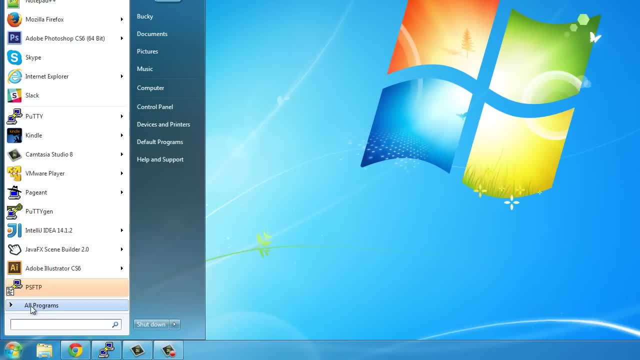 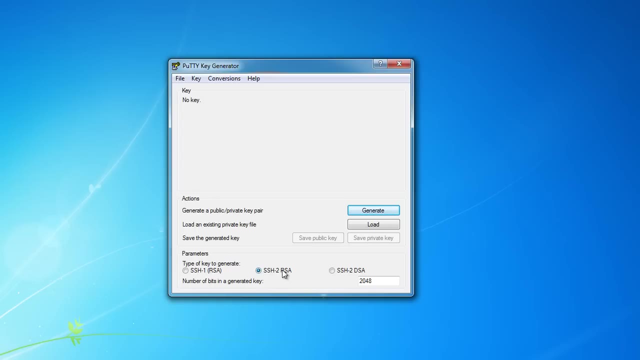 Well, check this out. There's actually a program that came with- if I can find it, Putty, called PuttyGen. So again, go to start Putty, PuttyGen, and this is a program to generate keys. So what type do you want to generate this SSH? These are just different algorithms or formulas, but the one that we want to use is SSH-2RSA. It should be there by default And if you hit generate, then it says: 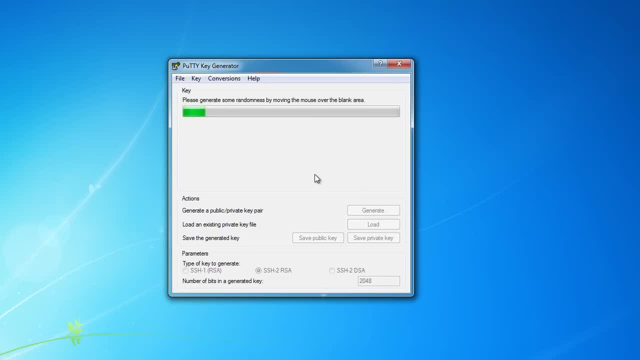 OK, This is a random key that's going to be unique to each user. So, in order to give it some random numbers as a seed, you just move your mouse over here- I don't know, maybe write your name, maybe draw a picture of you know, whatever- And then it says: OK, here is your random key. So, again, this is the public key that you see right here. This is what we're going to be sticking on the server, So select this. 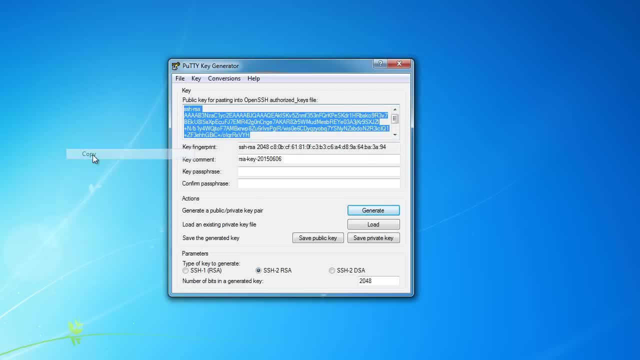 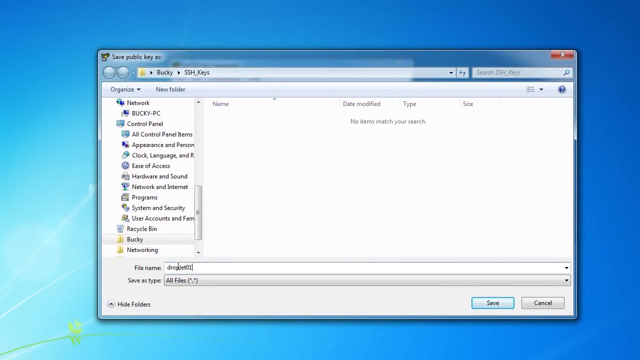 Select this all and just copy it, And then eventually we're going to be pasting into that terminal whenever we set everything up. But for right now let's just go ahead and save both of these keys on our computer. So whenever we close out of this, you know we don't have them lost. So I'm just going to save the public key, as it doesn't really matter what its name. So droplets 01- public. And you always want to save this as a text file. 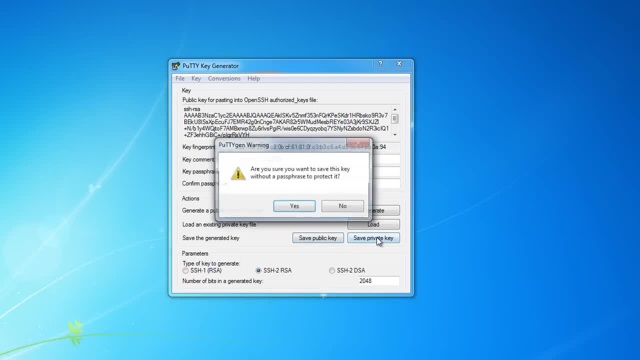 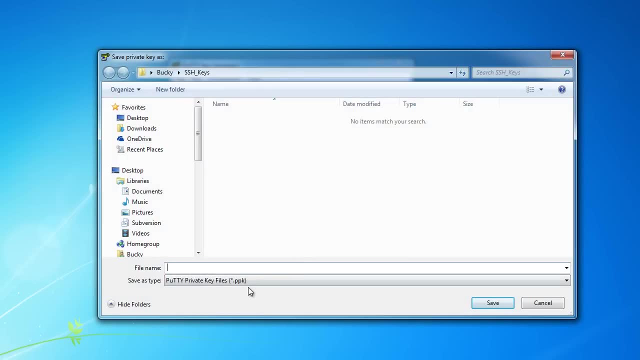 Dot txt, And whenever you save your private key, you usually want a password to protect it. But just for this tutorial I'm just going to skip it. Hit yes, So these private keys. they are stored as a special file, a PPK file. So I'm just going to name this droplet 01 private. 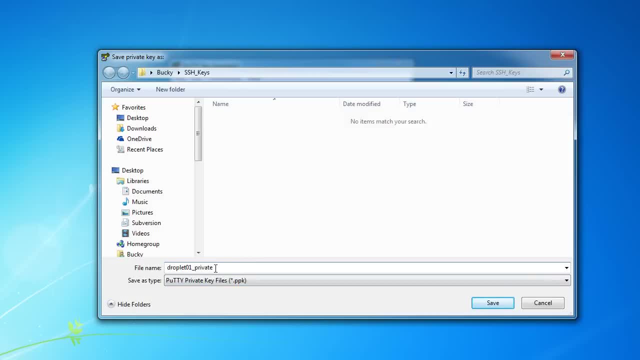 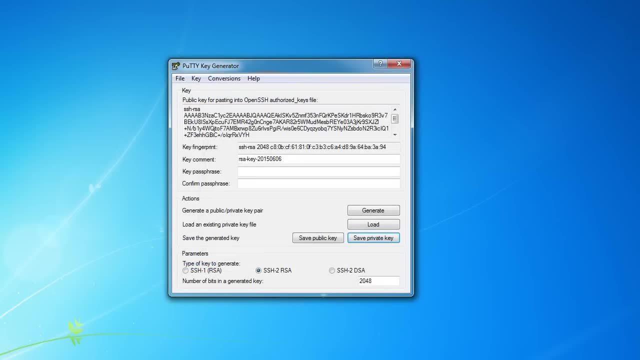 So now I have droplet 01, public and private keys, both stored on my own computer. But again, the only one that you really need is your private key and the public key. You just stick on the server, but you know, just in case. 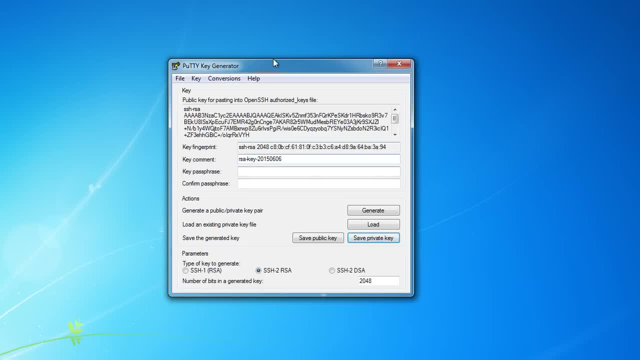 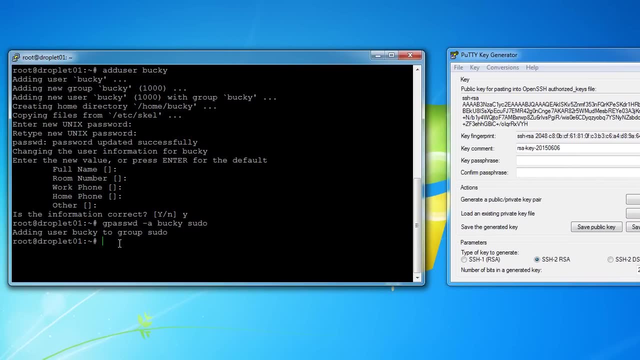 I lose anything, I want to have it backed up. So now that we got both our keys generated, let's just open up putty again and add that public key to the server. So the first thing I'm going to do is actually SU, which means switch user. 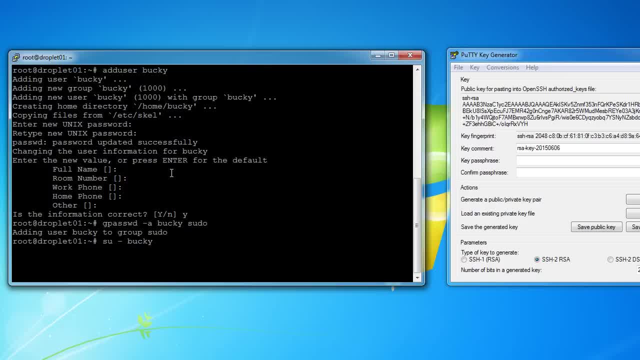 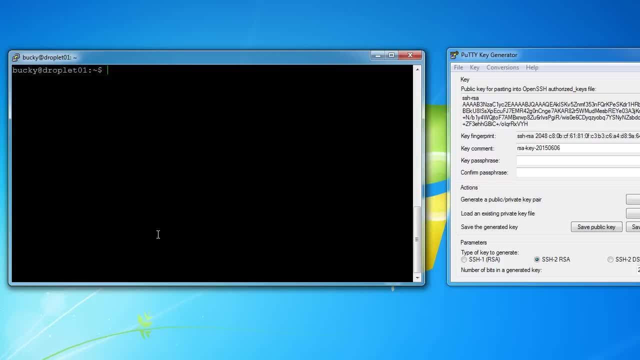 space minus space Bucky. So I'm going to switch from root to Bucky And I also want to clear this screen because it's getting a little bit, you know, jumbled up. all right, so you have to put these keys in a very specific. 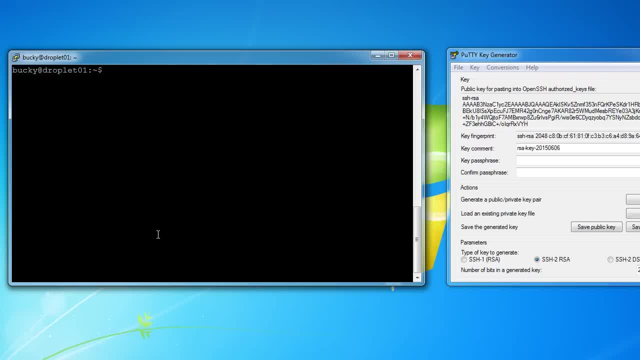 directory in that directory. it doesn't exist on our server by default. since this is a brand new server, it barely has any files on it. so mkdir, this means make directory. what do you want your directory or folder to be named? well, dot ssh, and you have to name it. this you just can't name. 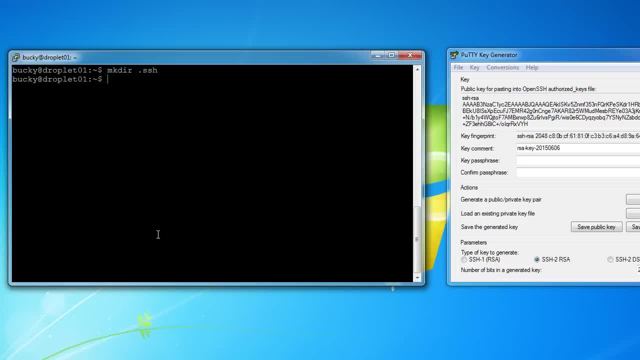 anything you want. so we now have a folder called dot ssh on our server and now what we want to do is we want to give it the proper permissions. so to change the permissions. that's a kind of change the permissions of a directory you ch mod and then you give it a special code. 700 means that 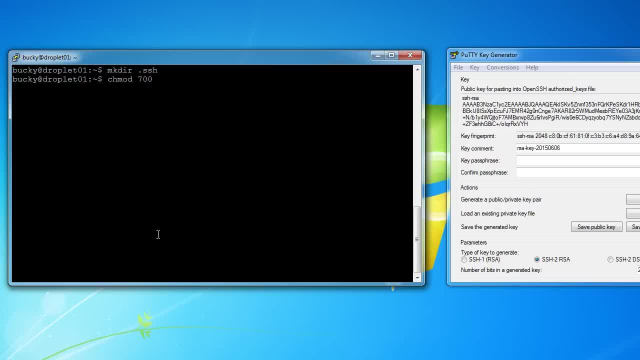 owners can read, write and execute from the directory ssh. and, by the way, any issues that you have with the directory, you can just type in the directory ssh. and you can. and, by the way, any issues that you have with the directory you can just type in the directory ssh. and 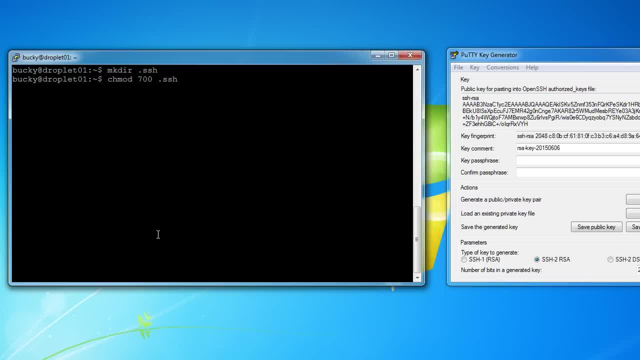 time you're trying to edit permissions for a directory, just look online at all the special codes. you don't have to memorize them all. so I know that this one is 700 hit. enter now. after this, we're gonna add a file in this directory and this is where we're gonna be writing all of our 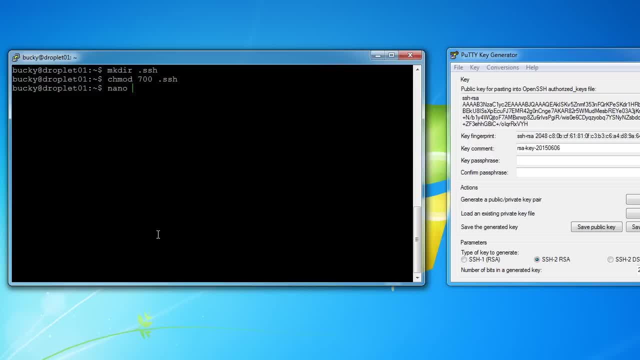 keys. so nano is I don't even know. it's like a text editor that's built into the terminal. it's the ugliest text editor you've ever seen, but it's the easiest way, so I'm gonna show. it's not. it's like worse than notepad, since it's all. 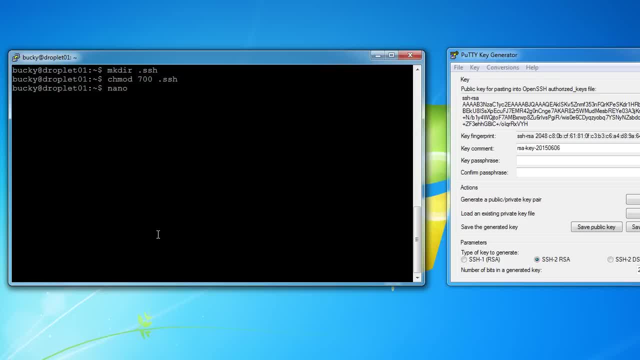 like through your editor. but whatever. so what file you want to open in this little text editor, if you can even call it that ssh minus authorized underscore keys, let me make sure that spell property authorized. looking good. now hit enter and there you go. look at this beautiful text editor. we. 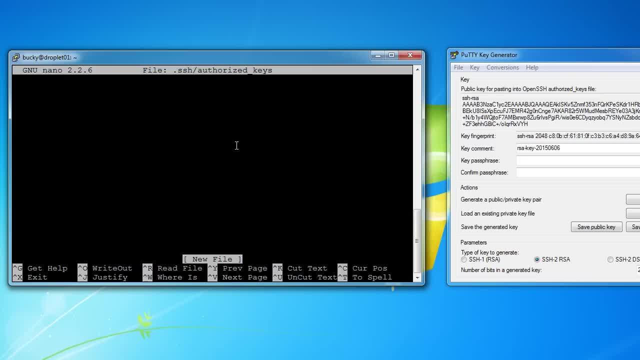 have. so all this file is going to do is gonna store the public keys. so remember, we already copied this, this public key. so if we just paste it in using shift insert, we're only gonna see the end of it because it's this long string, but the entire thing is pasted in. so once we have our data pasted in our 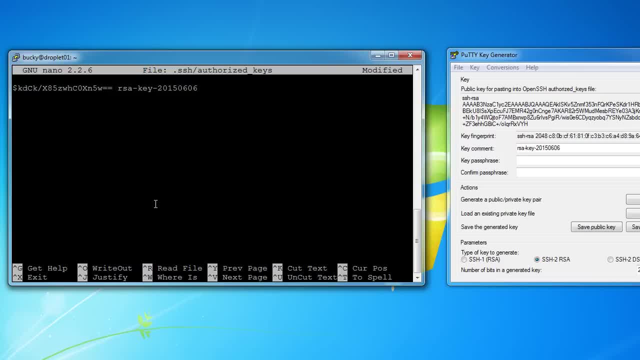 public key. just hit ctrl X and that exits this. now, before we exit out of this text editor saying: do you want to save the data that you just entered? hit Y for yes and then hit enter to confirm it. so again, whenever you made some changes and you want to save it and then come back here, ctrl X, Y and then enter. all right, pretty cool now. 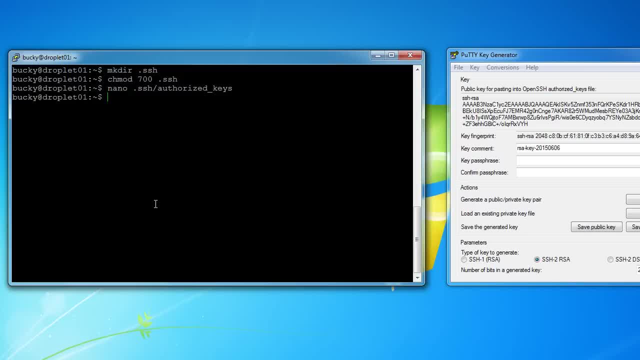 the last thing we have to do is this: we already set up our permissions for the directory, but now we want to edit the permissions for that authorized key file and we want to do this so the owner can read and write to it. so ch mod: this is 600, 700 is if you want to execute them to. 600 is just for. 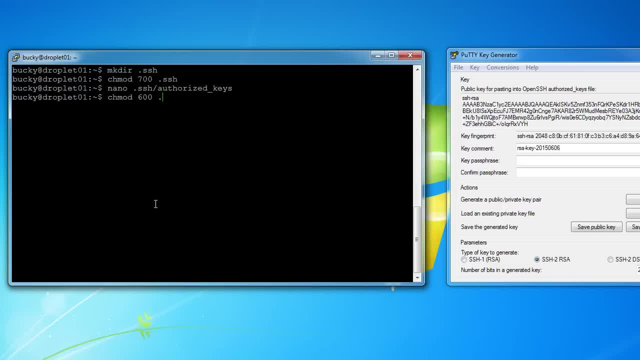 reading and writing without executing. so again, that's dot, ssh, authorized underscore keys and hit enter. so now we have our public he set up. so what this means is that whenever bucky locks in, he's going to pass in his private key, it's gonna look at the public key that's already in there. and if everything, works out, he's going to be able to connect to the server. all right, pretty cool, so you can actually close out of the server. terminal inside the server gets closed. server is ready now, after you've already adapted that interface into restart, something like this: you just click call refinder and uma flower and then we'll be able to open this up here. community manager, and let's do this. 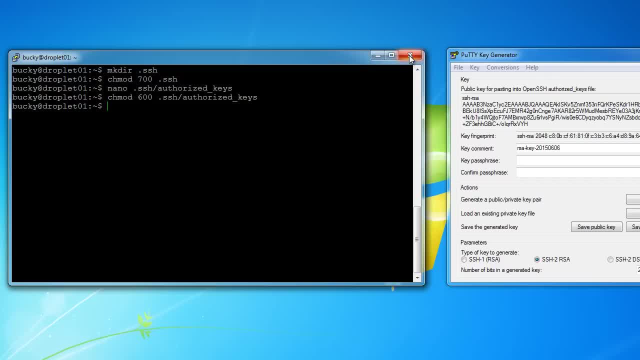 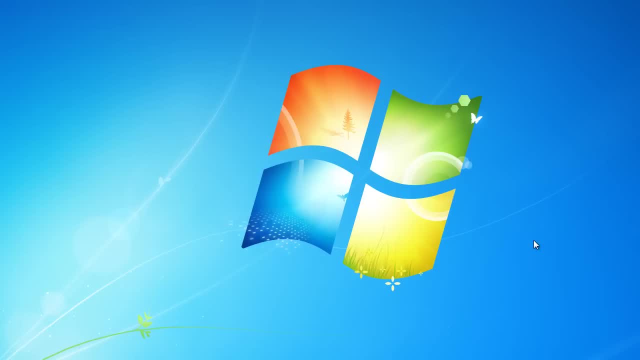 Alright, pretty cool, So you can actually close out of this. Are you sure you want to close this session? Yep, And we can actually close out of this as well. So you may be wondering: alright, whenever I try to connect to the server, how does it know where my private key is? I know where I saved it, but how does my computer know? 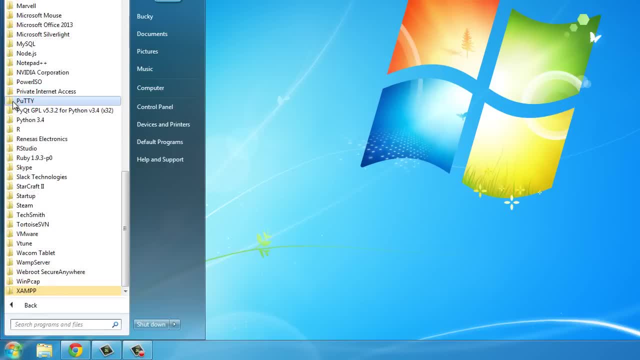 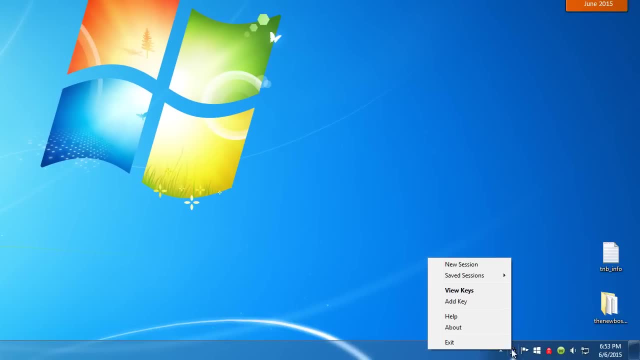 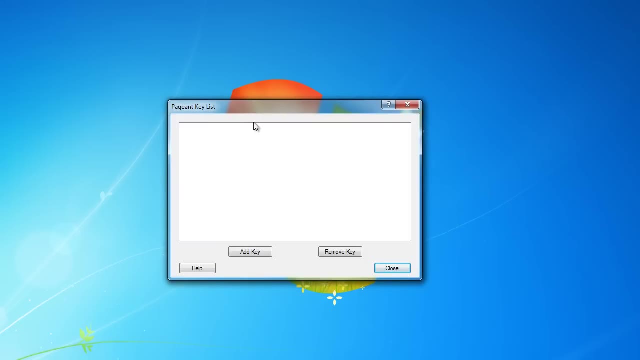 Well, actually, if we go back into all programs putty and open up this program P-A-G-E-A-N-T- I actually already have it running, So I just got to click right click it and view keys. This is your SSH private key manager, So whenever it tries to connect using SSH, it's going to look here for all of the keys.